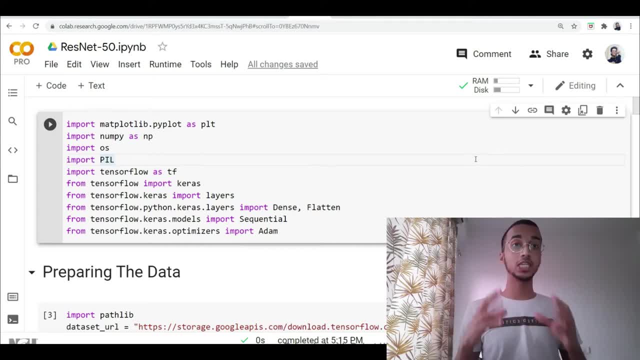 Hello everyone, my name is Nachiketa and welcome back to another video. In this video, I'm going to show you how you can implement the Keras library to implement transfer learning on any of your image classification problem. I have previously made a video on this using the VGG19 model. In this I'm going to show you how to do it using the ResNet50 model. And in this video I'm going to be using a much simpler code and I'm going to guide you through the complete process: from obtaining a data set, preparing the images, giving it to a model, how you can exactly fine tune a state of the art image classification problem. 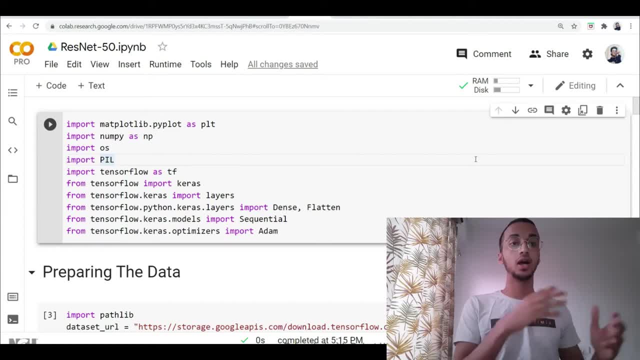 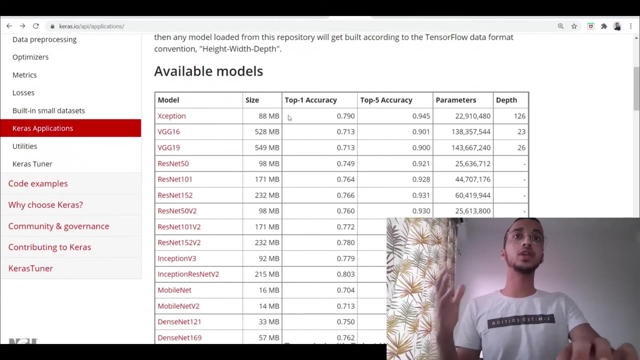 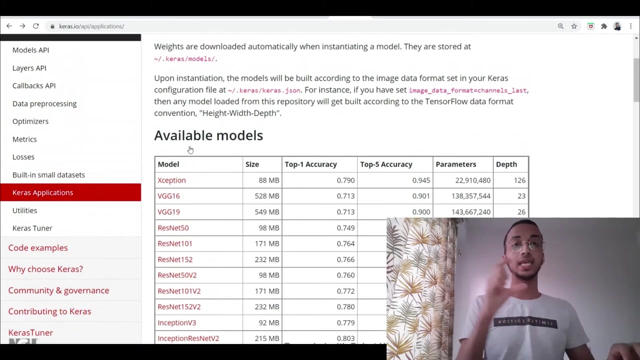 And, finally, how to evaluate the model, visualize its metrics, as well as make predictions on new data. So I'm going to guide you through the complete flow. So let me just first give you a gist of what transfer learning is. So what Keras has done right. it has made available state of the art neural networks like Exception, VGG16, ResNet50. And all of these models have been trained on the ImageNet data, which basically contains millions of images. So, whatever this model, 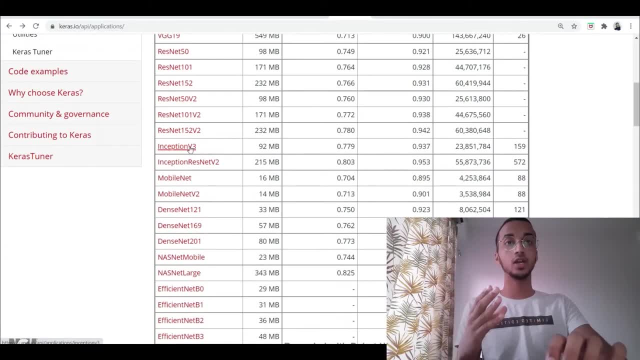 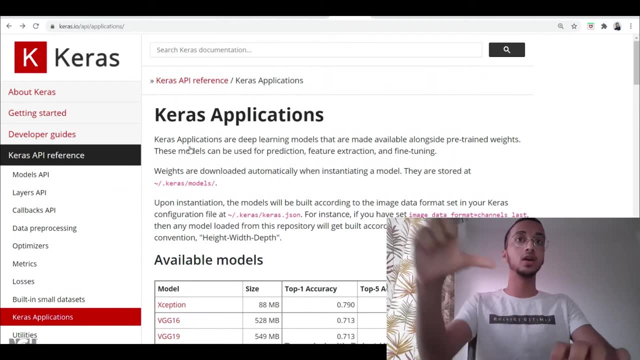 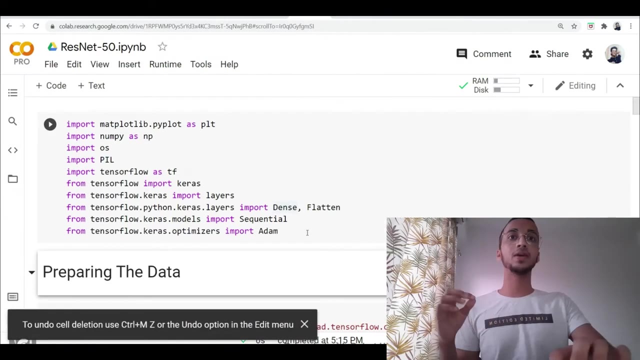 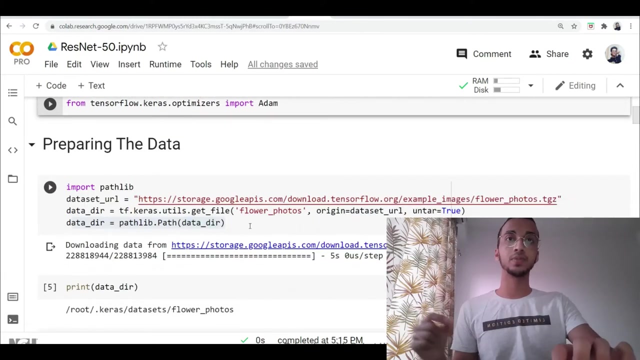 has learned. all of the weights can be transferred and used for your own image classification problem. That is why it's called as transfer learning, because you're basically transferring the learning of these models. So let me just show you how we can implement it and you'll understand it as we go through the code. So the first step is to import all the libraries. I'm going to explain them when we come to them in the code. So, of course, to start with, you need a data set So you can have your own data set, But for now I'm getting images from this TensorFlow URL of: 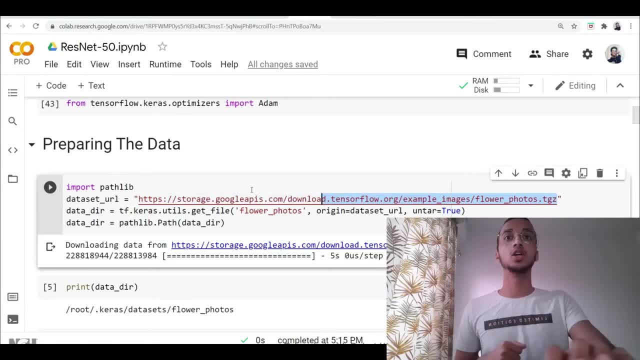 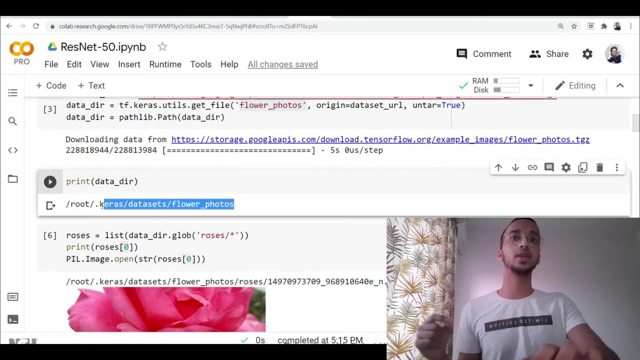 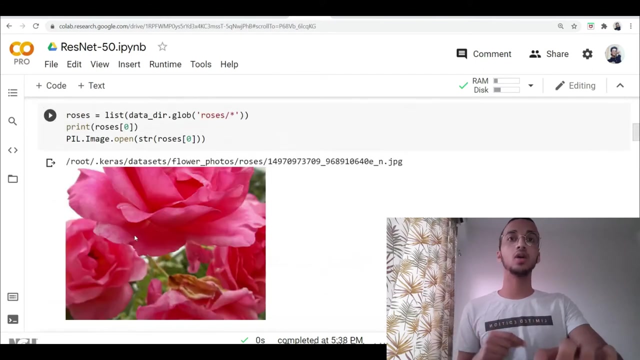 flower photos, which are basically images of different types of flowers. So in this line, I'm basically fetching data set from the URL that I mentioned and I'm saving it into a folder called as flower underscore photos, And if I print the directory, you can see that the data set is going to be stored over here. And now let me just print and show what kind of an image we're dealing with. So this is how a rose image looks like. So the only thing you need to execute this code is a folder of images. 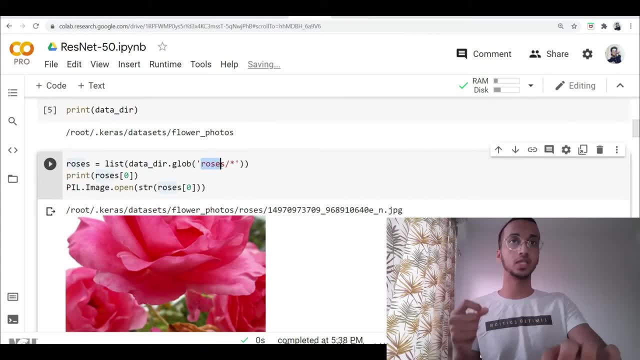 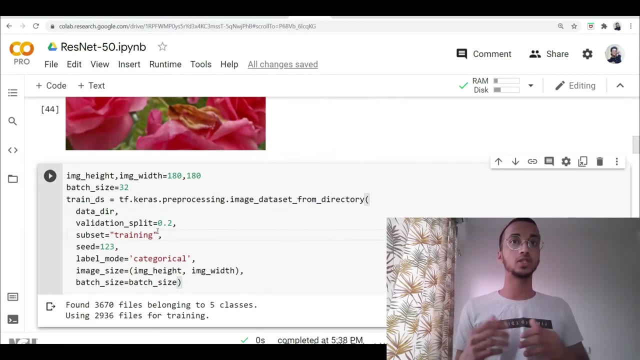 So in the flower underscore photos there's a folder by the name of roses. Similarly, there's going to be a folder for each class of flowers For your data set. make sure you have a folder of all the images. Once that is done, here's where we're going to be splitting the data set into training and testing and doing some other pre processing. So we use the image underscore, data set underscore from directory class, And what this does is it takes the directory of the images And here you can mention what should be the training and validation split. So right now, 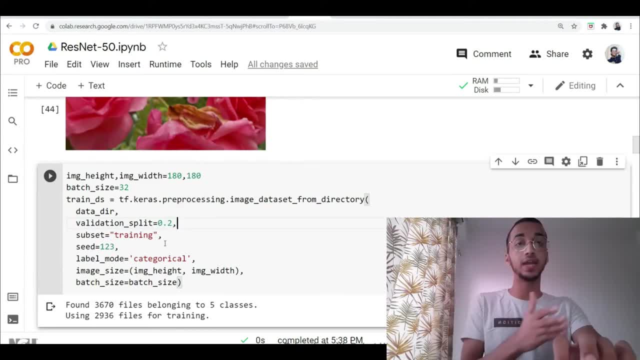 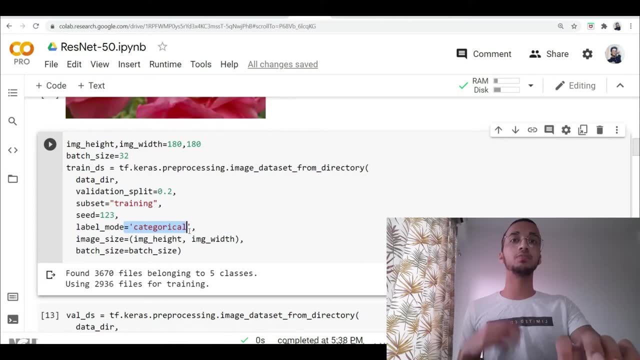 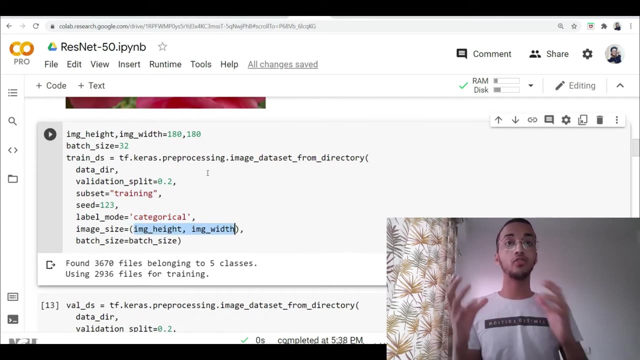 what's going to happen is 80% of the data is going to be used for training and 20% for validation. Here I mentioned that the first subset is going to be training And when I write label, mode is categorical. basically means there are different classes and categories of classes And you have to mention the image height and width. So in your folder there are going to be a lot of images and they can be of different dimensions. So what I've done is all the images are going to be resized toward dimension of 180 cross 180.. You can change it to any dimension you want, And I've also 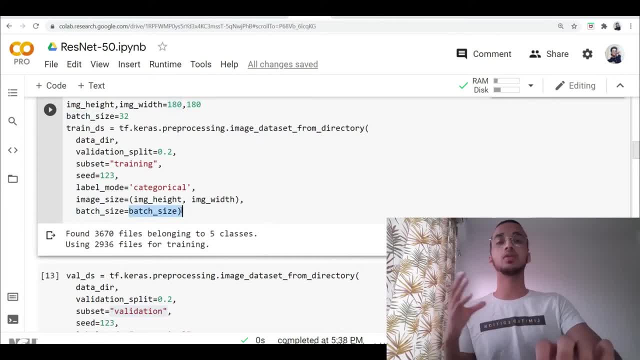 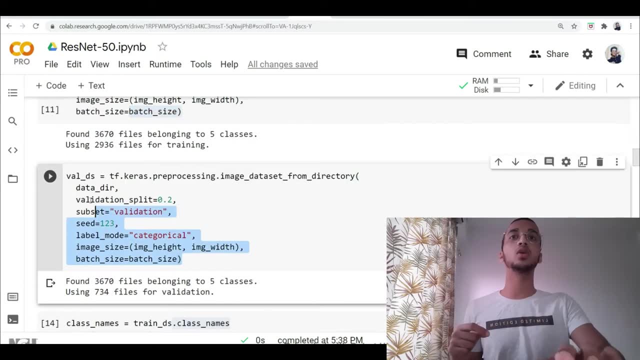 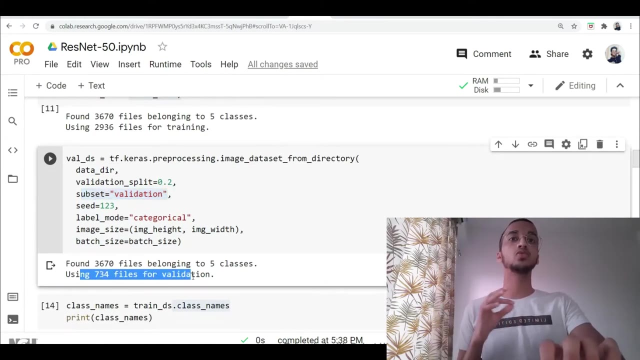 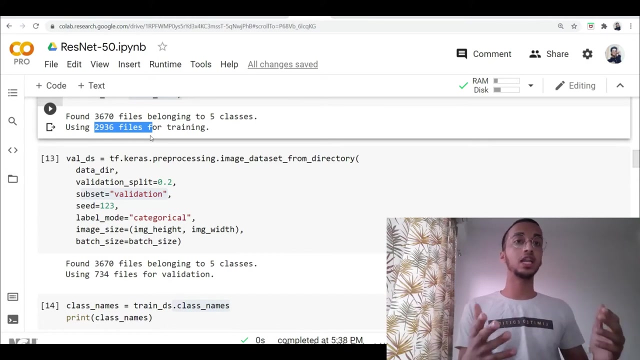 specified the batch size of 32 over here. If your system has a lower RAM, you might want to reduce it to, let's say, eight or four. Similarly, the same code for the validation part. the only difference is I'm mentioning the subset as validation And you can see that around 734 files are being used for validation and 2900 files are going to be used for training. So the splitting into training and validation is automatically going to be done for us. Now I am just printing what are the different classes in. 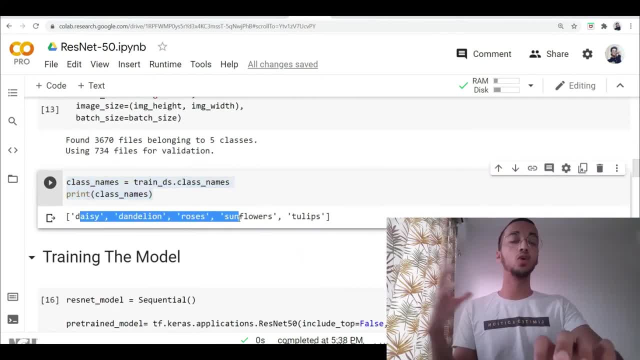 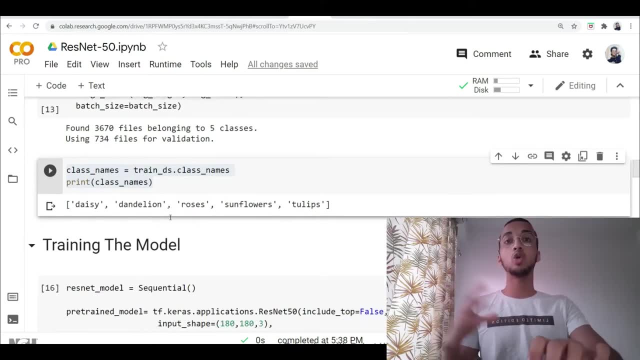 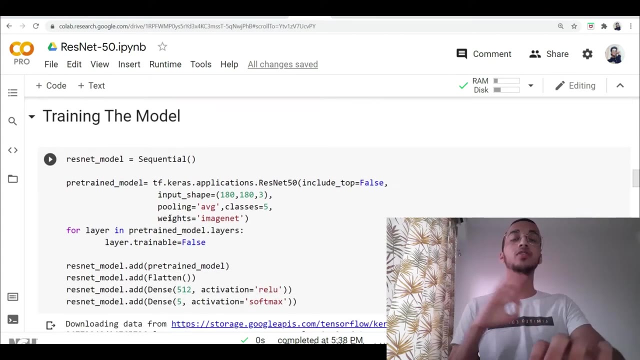 inside my data set. So these are basically the names of all the folders in my data set. So there are five classes of flowers and my model has to learn to recognize all five. So how do we exactly get state of the art models And how do we fine tune into our model? Here is where that part comes in, And this is going to be very simple. First, what I'm going to be doing is I'm going to be creating an empty neural network. I'm initializing by calling the sequential function, And this makes sure that the layers that are going to be added are going to be added in a sequence one. 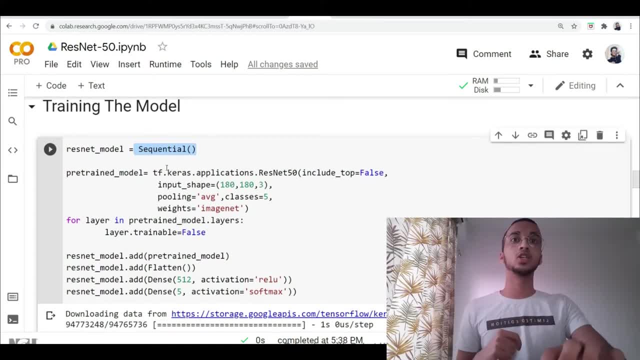 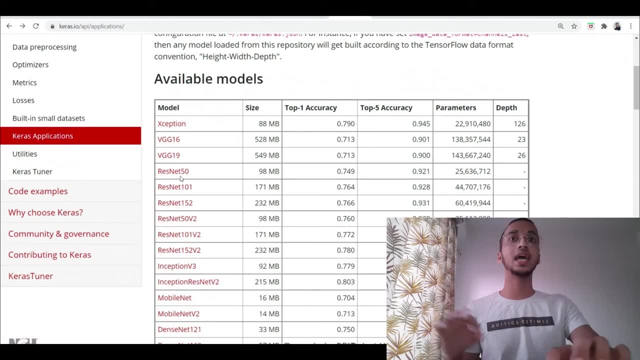 after the other. so how do we get resnet 50? so this is the code that does that. and where did i get this code? it's very simple: simply go to keras applications documentation and click on any model you want. so let's say, i clicked on resnet 50 and it gives you the code to import. 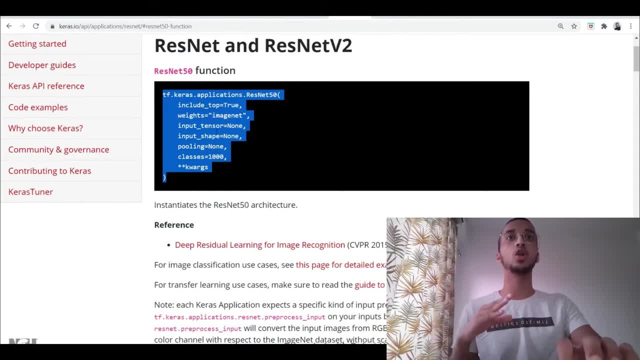 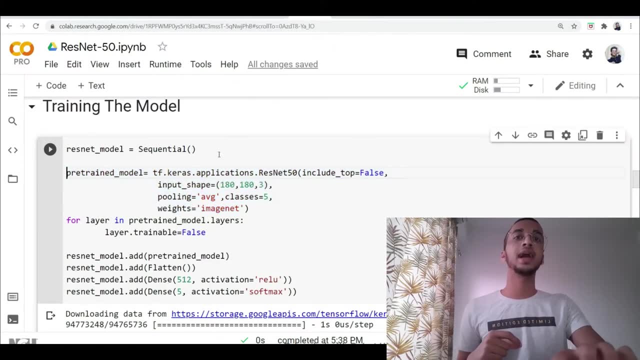 the model, all right. so simply copy this and paste it. if you want to use some other model- exception inception- you just have to do the same thing. so here is where i copy that part of the code and i'm giving it the name as pre-trained underscore model. and there are some important. 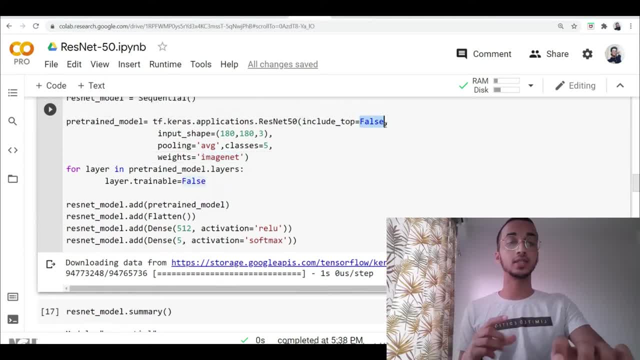 things over here. include underscore. top equals to false. this basically means that i'm going to be using my own input layer and my own output layer. why did i do that? because the original resnet model might have been trained on different image dimension. my image dimension is different. 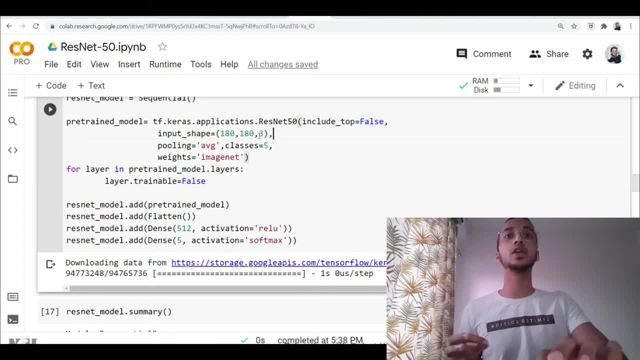 so that's why i write this parameter as false. and over here you have to mention the input shape of your data- number of classes- and you have mention the type of pooling- it can be average or max- and which weights are you gonna be using. so weights- that was learned by training on the ImageNet problem. that is, the weights. 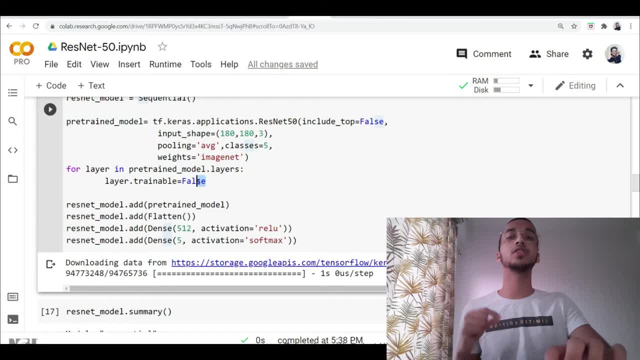 that I am gonna be using. alright. so here I mentioned that for layer in pre trained underscore model, which means that every layer inside that pre trained model is not gonna be trainable, because I am writing, trainable is equal to false. so basically means that whatever the ResNet Model has learned, do not learn those weights again. keep those weights as it is. 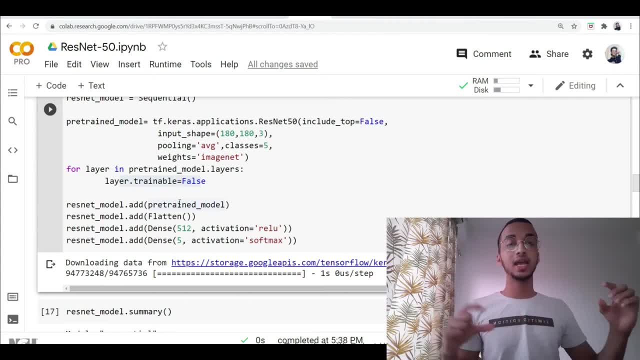 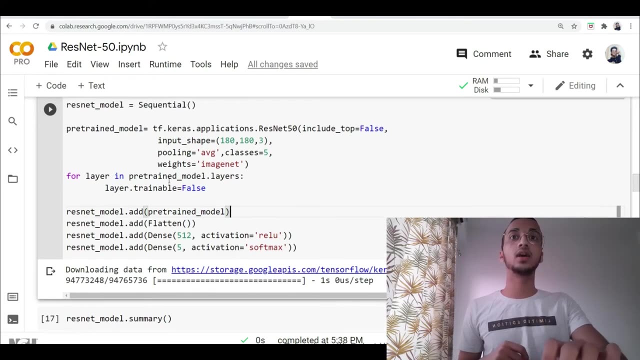 I am just gonna be adding my own input layer, my own output layer, and there the learning process is gonna be done. but whatever the ResNet model has learnt, that is not gonna change. this basically saves a lot of time, complexity in the training process. so now what I am gonna be doing is I am gonna be adding this pre-trained model to ResNet model. that I had created over here. so now I am basically flattening this pre-trained and then I am creating a model that is going to be used. whatever model I can sketch, and in the next few days, as any. these examples, as I get used to them. 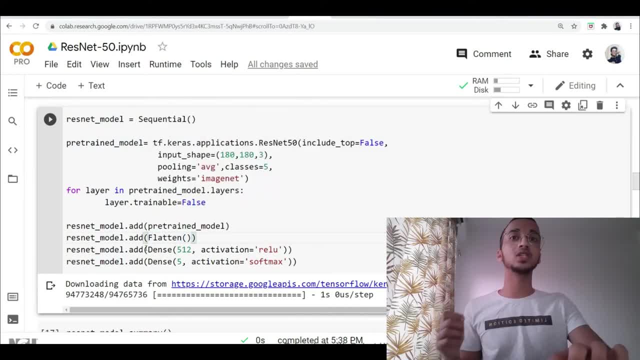 whatever the model gave it- into one dimension, and i'm using some fully connected layers at the end, so you can add three, four layers if you want. so these 512 neurons that i'm adding, these are the ones that are going to be learning the new weights, right? the rest of the weights in the hidden layers. 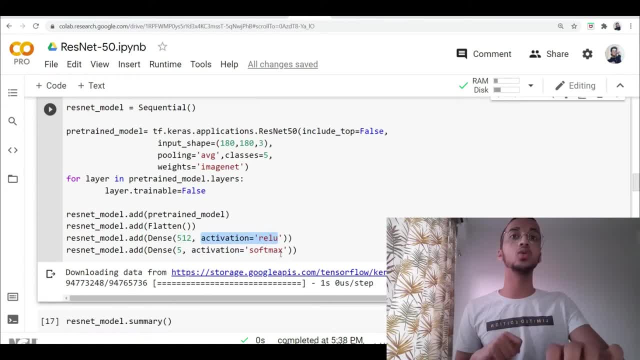 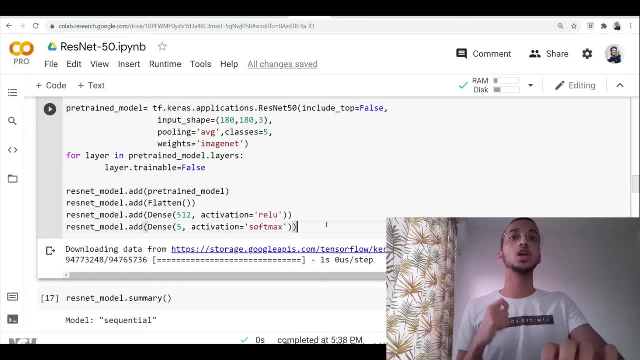 are going to stay the same and i've mentioned the activation function as relu and the final output layer has five neurons because there are five classes and the activation function is softmax. so once you run this, it's going to download the model from the cadasa application and over here. 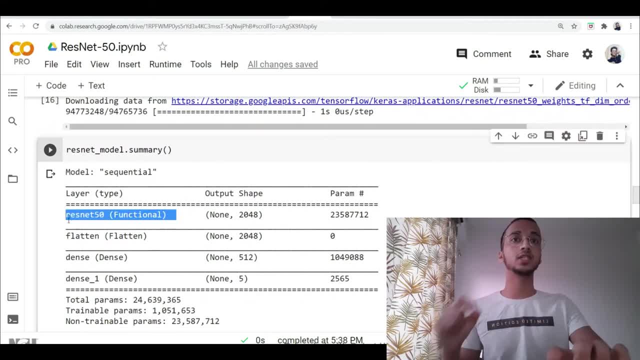 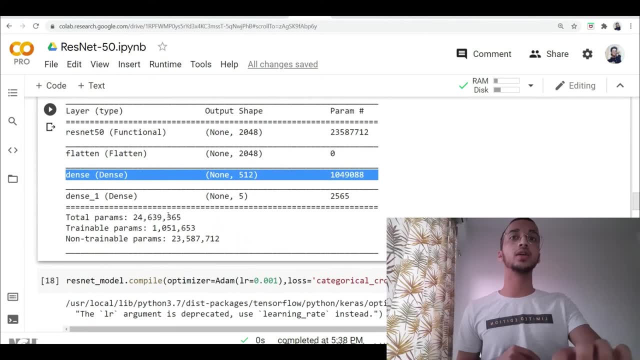 you can see the summary. so initially we have the pre-trained resident 50 model. to that we added our final fully connected layer of 512 neurons and you can see the effect over here. this was the total number of parameters and these are the trainable parameters. rest of the parameters: 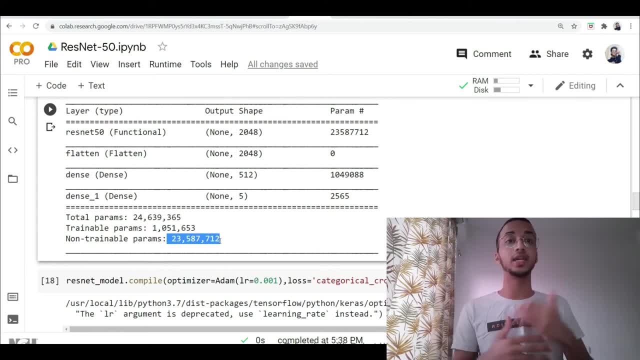 are non-trainable, right, because model is not going to learn that again, because resident 50 has already learned it right. so we don't need to do the training again for those hidden layers now. once your model is ready, you simply have to compile it. you have. 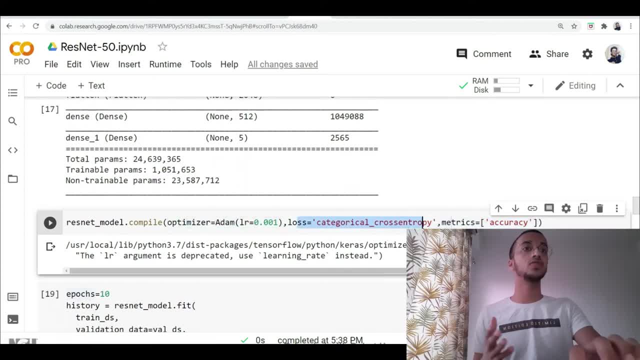 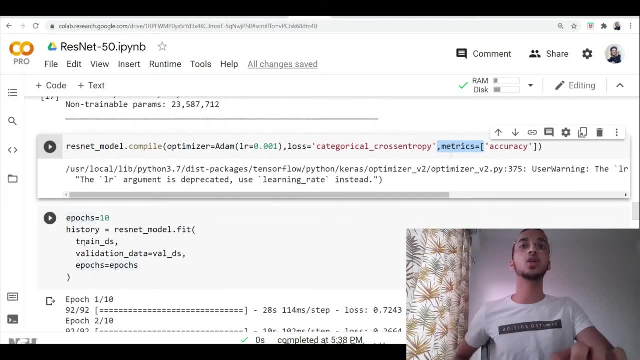 to provide it one optimizer. i'm using adam, i'm using a loss function of categorical cross entropy and the matrix is going to be accuracy. once you run this, you simply have to fit the model, you have to provide it the training data set and the validation data set and you have to specify the 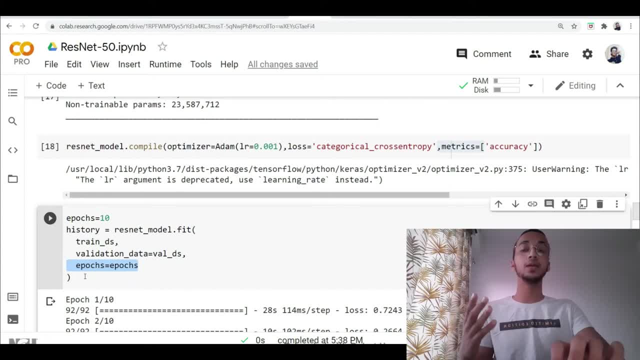 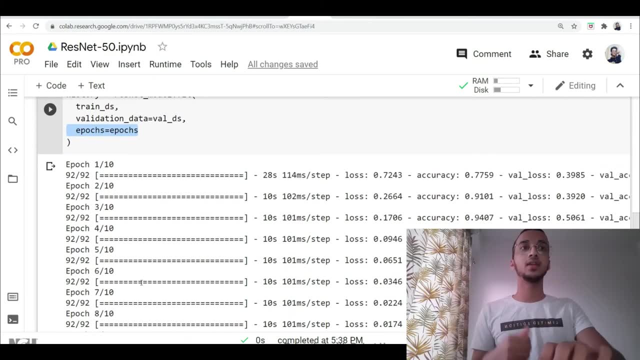 number of epochs and i noticed that i only needed 10 epochs for a good accuracy, but you can increase that number as well. so i have already trained the model and i'm going to show you how to do that. i'm not training it again because it takes some time, but you can see that with different epochs, the 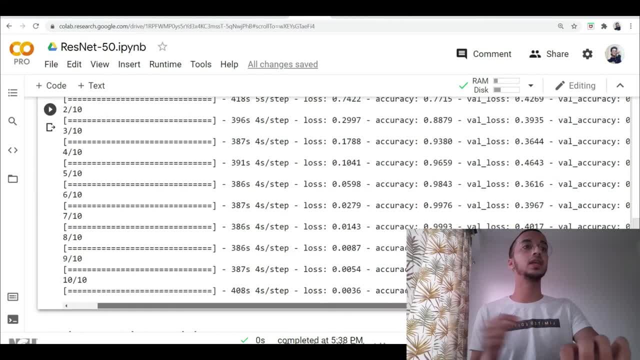 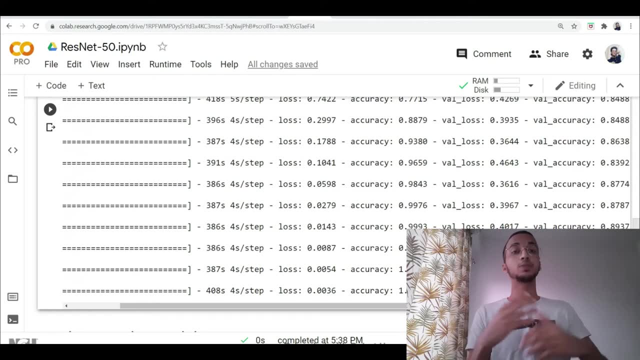 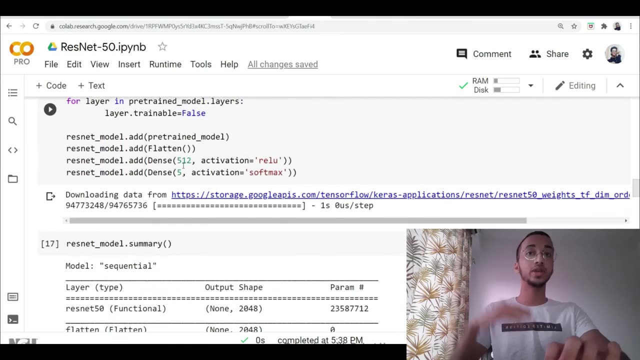 accuracy was increasing and it seems to have overfit a little at the end, and the training accuracy is 100 and the validation accuracy is 88. and if you want to experiment with this, you can change the output layers. you can reduce the number of neurons from 512 to, let's say, only 64, or you can add 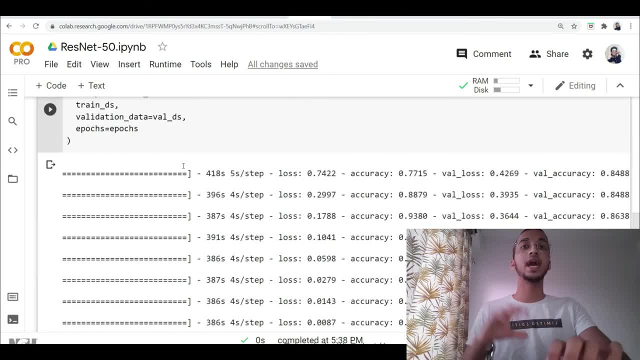 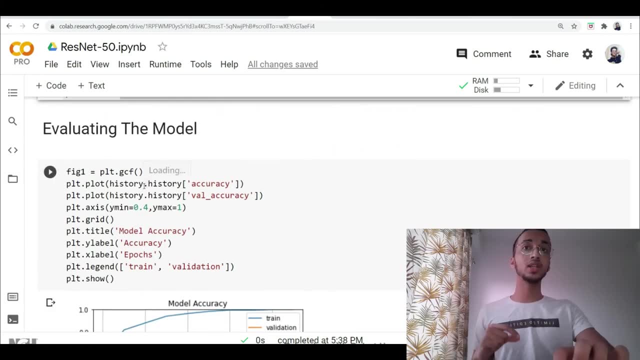 multiple layers as well. so that is for you to experiment with, and now let's visualize the output and the learning part of the model. so basically what i've done is i had stored the model's logs in a variable called as history and basically i'm accessing the accuracy and the validation accuracy and these lines just play the. 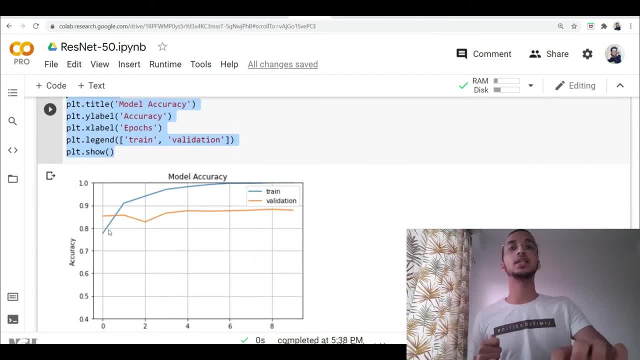 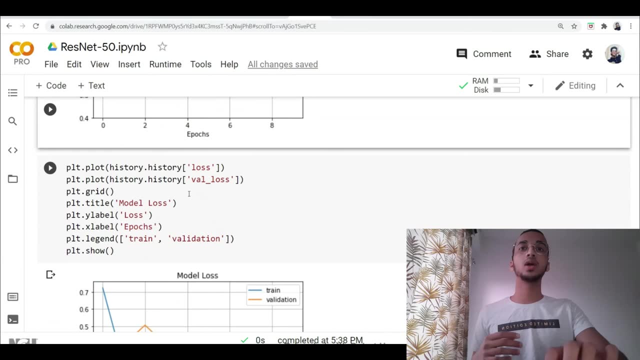 role of labeling the graphs. so once you run this you can visualize the uh training accuracy in the blue line and the validation accuracy. similarly, i'm going to plot the loss of the model as well. so the loss was declining somewhat for the training but for the validation it was not declining that.